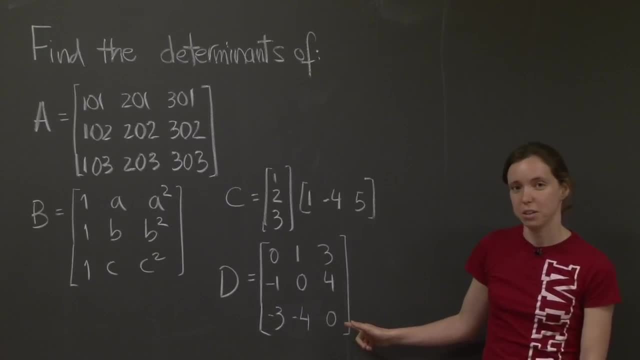 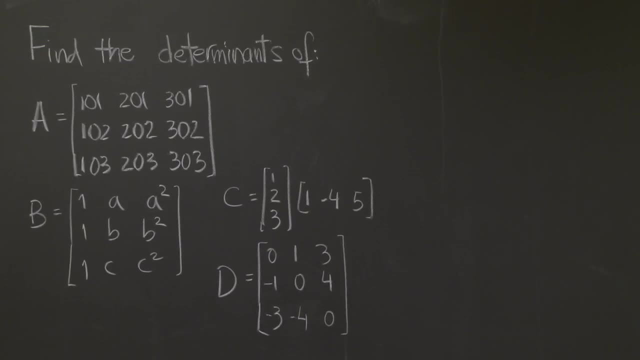 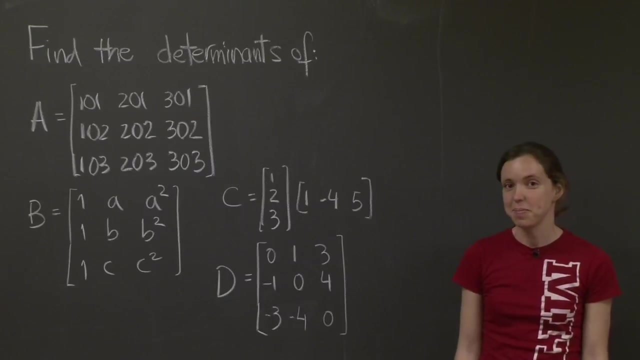 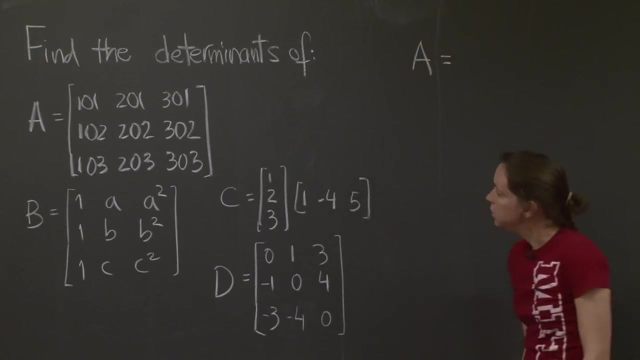 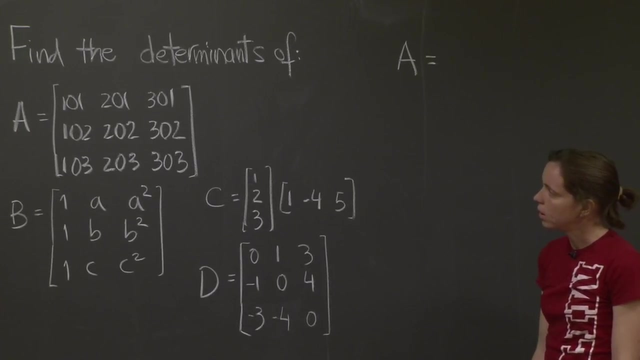 D. is this matrix? All right, Good luck. Hit pause, Work on them And when you're ready, come back and I'll show you how I did it. All right, Did you get something Awesome? OK, Let's do it. Start with matrix A. Well, I have lots of big numbers I suggest. 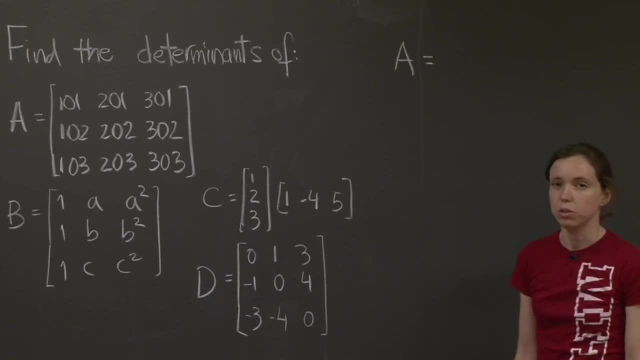 that we do a little bit of elimination, Because, as you know, doing elimination steps, except for permuting rows, doesn't change the determinant of the matrix. So let's do determinant of A. So I have this matrix, I'm going to write it down. I'm going to write it down as Vandermonde. 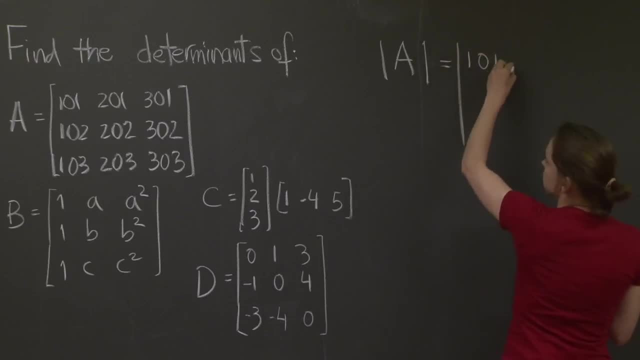 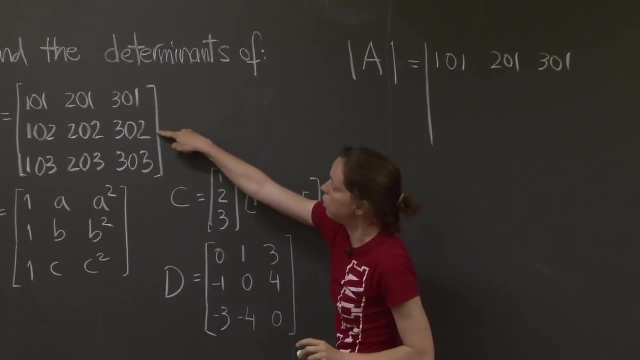 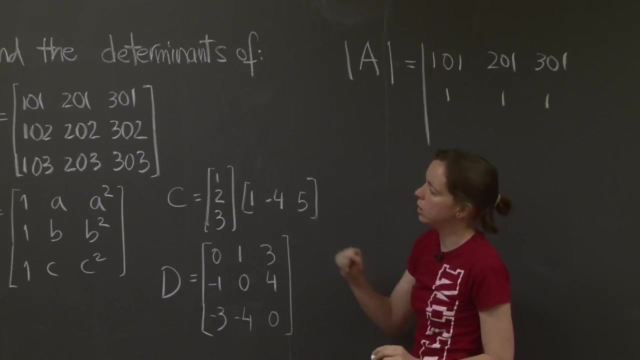 A is equal to 101, 201, 301.. Then if I subtract off the first row from the second one, I'll get 111, which is very convenient, And actually if you subtract the second row from the third one, you'll get 111.. Here's the property of the determinant If you have two equal rows. 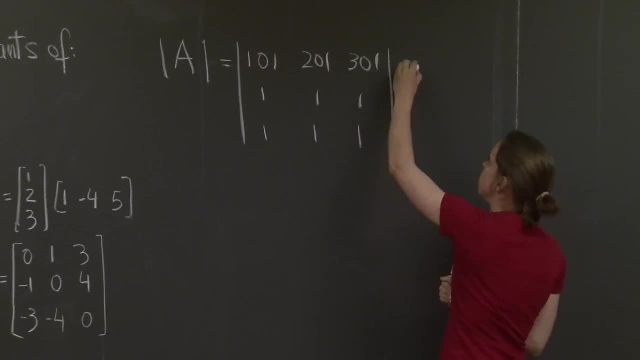 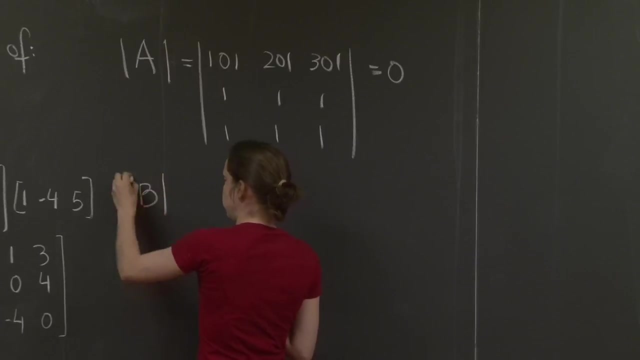 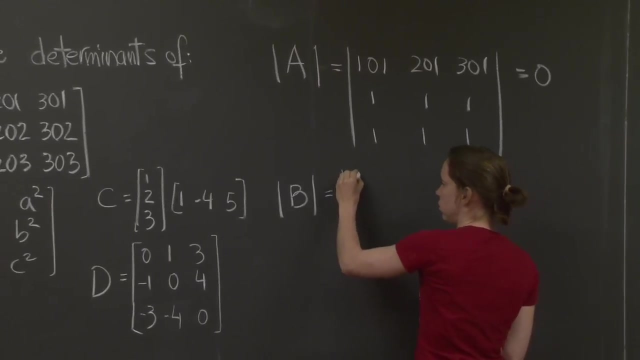 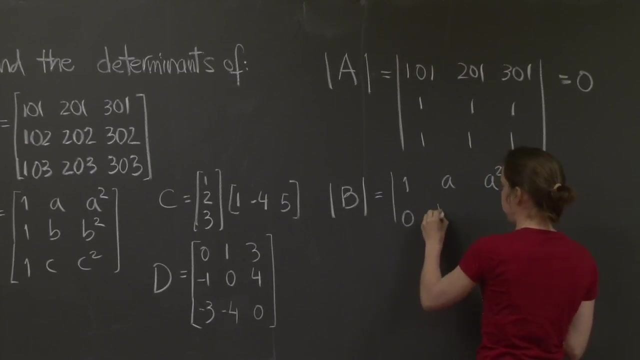 On your matrix, the determinant is automatically equal to 0.. All right, all done with one of them. Let's work on the second one. Determinant of B. Well, let's try elimination again: 1, a, a squared 1 minus 1 is 0, b minus a. 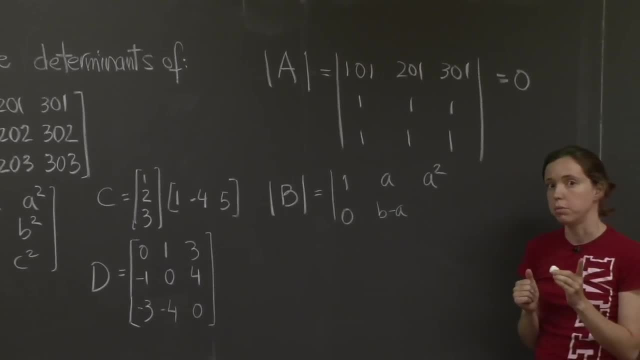 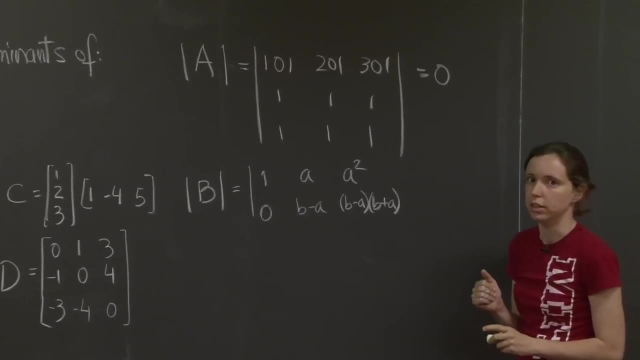 and b squared minus a squared. b squared minus a squared. let me factor that into b minus a, b plus a, which will be very convenient in the next step, And then I'm going to subtract the first row again from the third one. 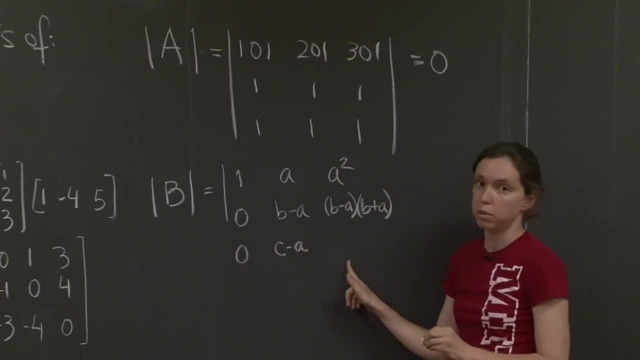 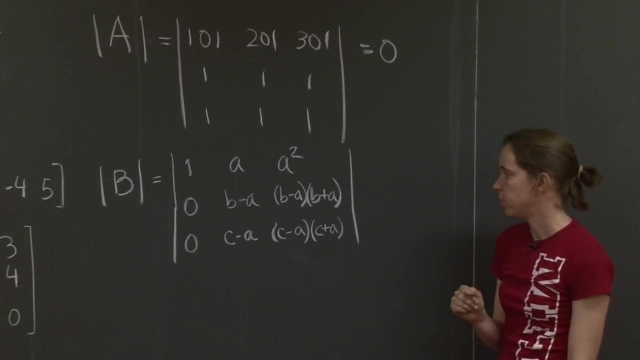 I'll get 0, c minus a, and again I'll get c squared minus a, squared c minus a, c plus a. All right, let's use that second property. third property: that was the determinant is linear on each row separately. 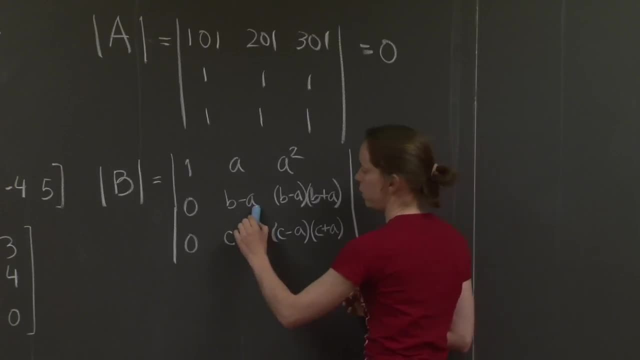 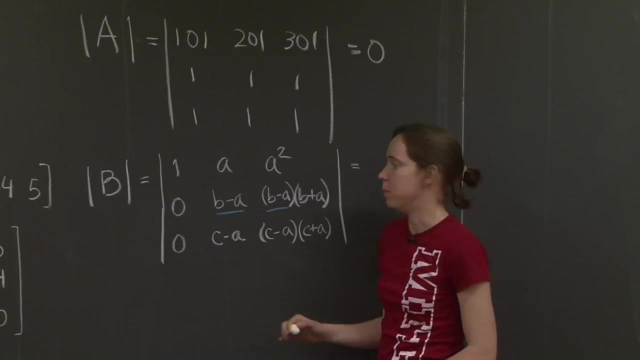 So what I'm going to do is see this factor of b minus a shows up in every entry of this row. Well, it's a 0, so it's the 0 multiple of b minus a. So I'm going to pull. 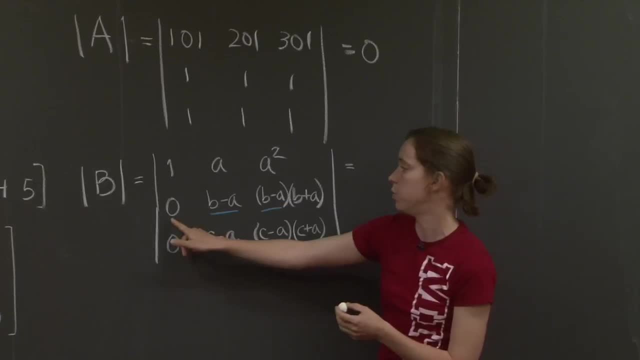 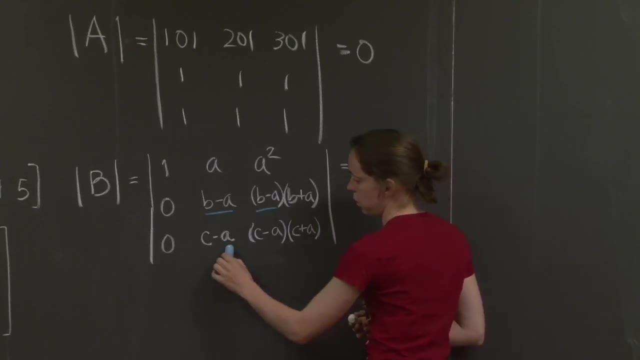 I'm going to pull out this factor of b minus a, and this row is going to become 0, 1, b plus a. I will also, in the same step, do the same thing with the third row: I'll pull out a factor of c minus a. 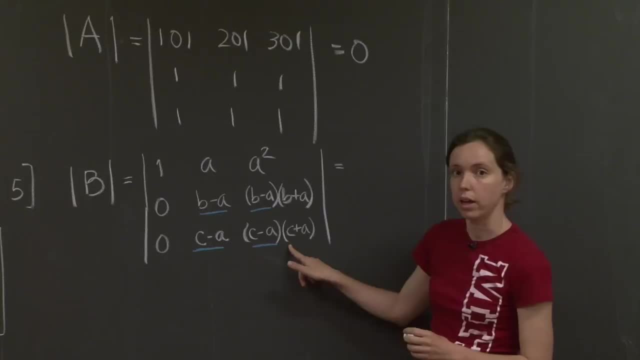 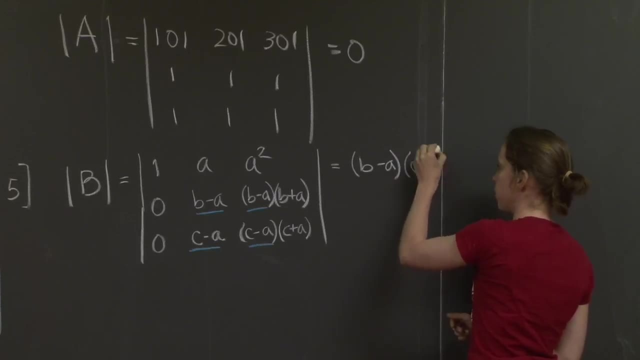 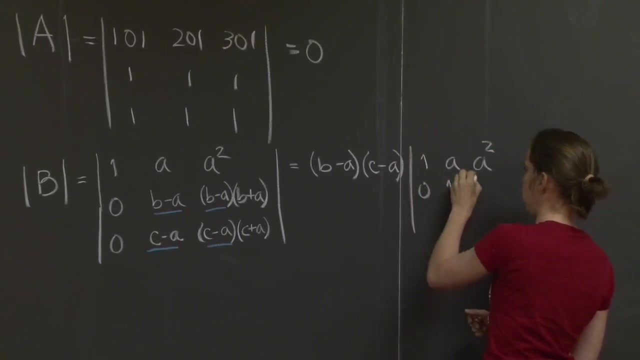 and it will become 0, 1, c plus a. Here's one factor from the second row, another factor from the third row, and 1, a c plus a. All right, So this is going to be a squared 0, 1, b plus a, 0, 1, c. 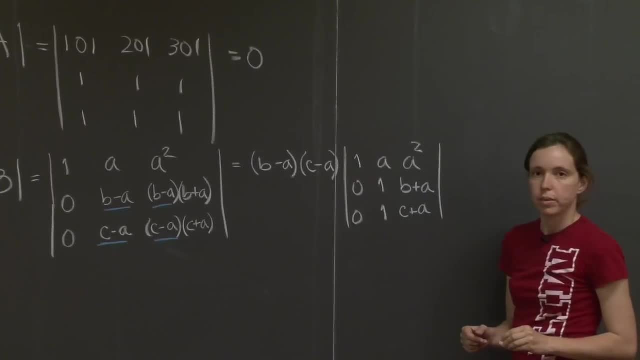 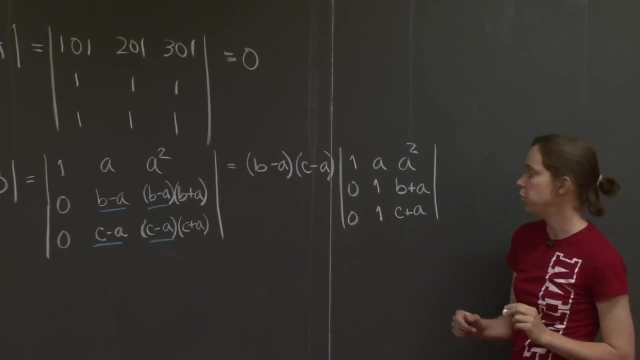 plus a. Now what? Well, remember, you know how to do the determinant of upper triangular matrices, because all that you do is multiply the pivots. This is almost upper triangular, except there's a 1 over here. So let's do another elimination step. 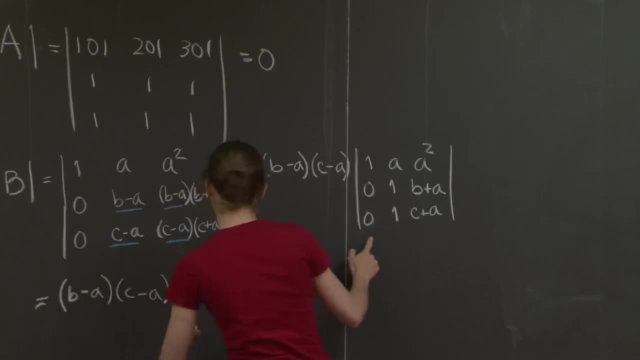 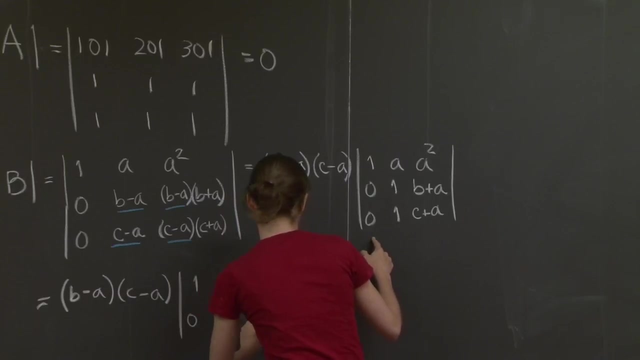 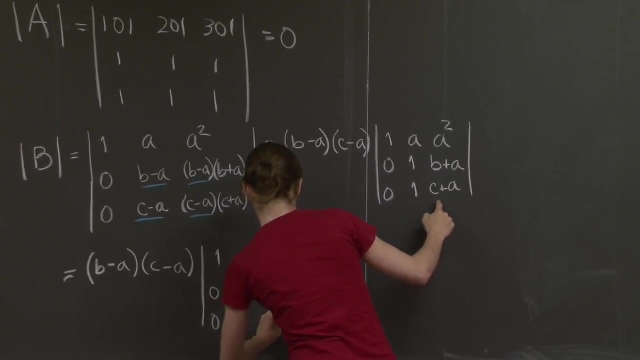 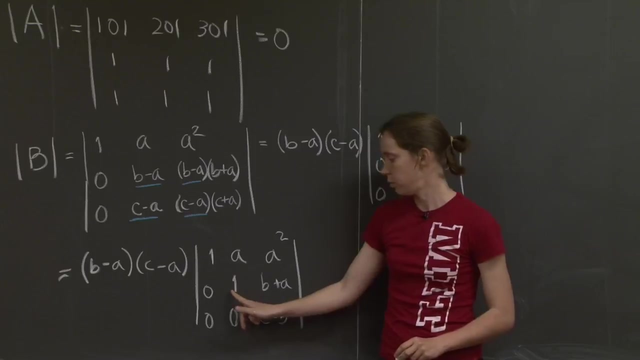 b minus a. c minus a: 1, a, a squared 0, 1, b plus a: 0, 0.. c plus a minus b plus a is c minus b. So the determinant of this matrix is now 1 times 1 times c minus b. 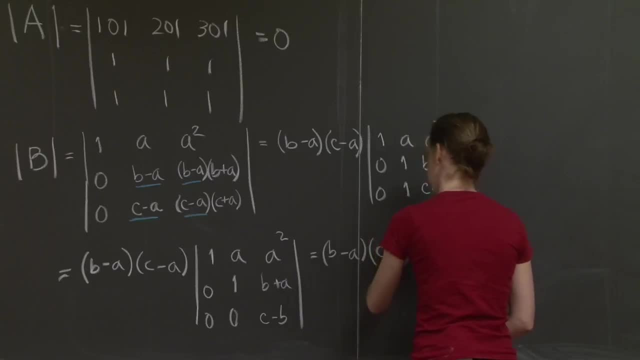 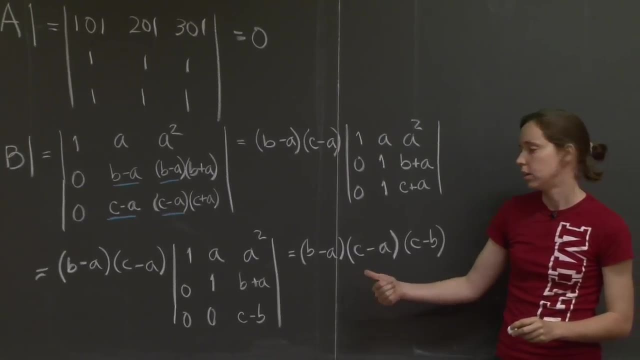 So we get b minus a, 1. c minus a, 0. b- 0.. c minus a, c minus b, Which has a really nice formula. This is called the Vandermonde determinant. It's always like this: 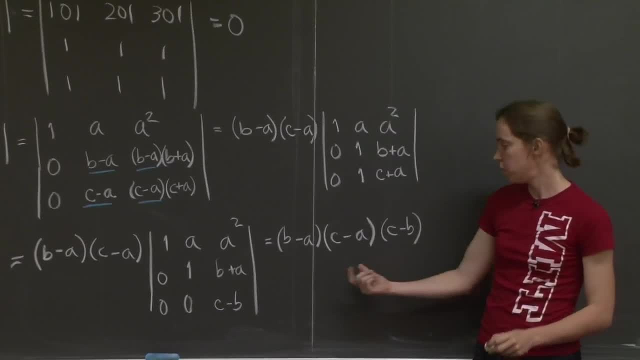 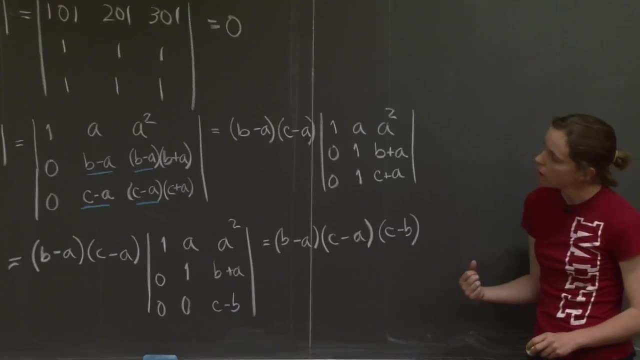 Even if your matrix is bigger than 3 by 3, if it's 4 by 4, or 5 by 5, and so on, you just have more differences of all the letters that show up in your matrix. On to matrix numbers. 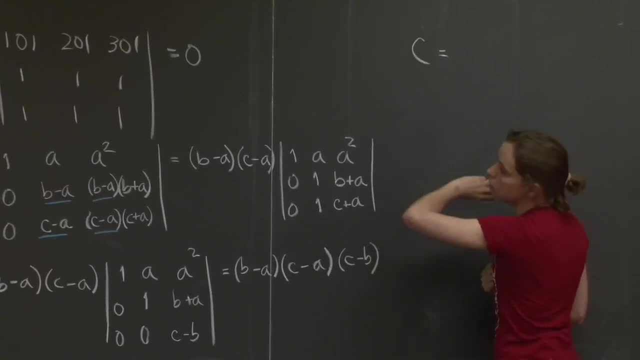 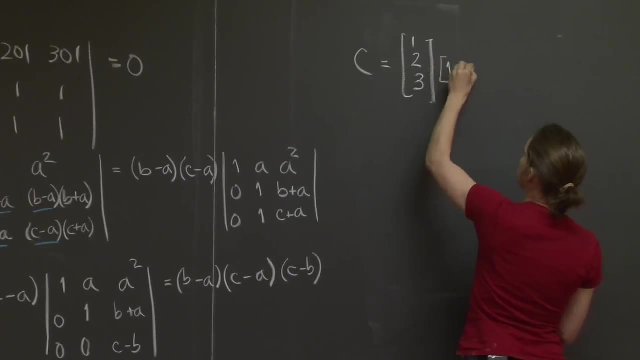 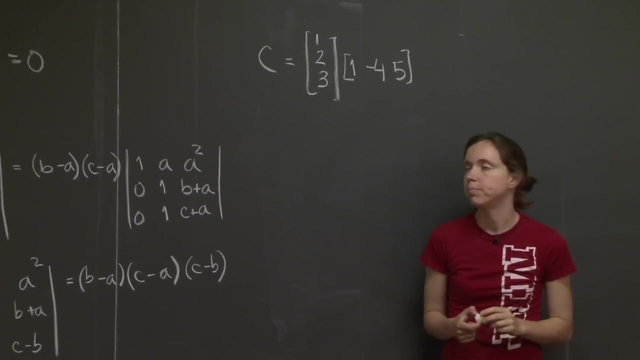 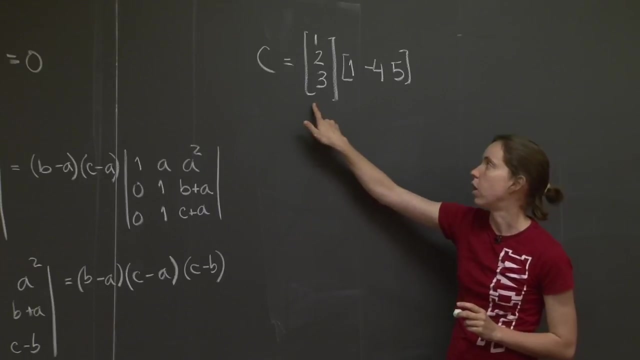 Number 3, c equals 1, 2, 3.. 3, 1, minus 4, 5.. How did you get the determinant for this one? Well, remember, this is a rank 1 matrix, because it's a column vector times a row vector. 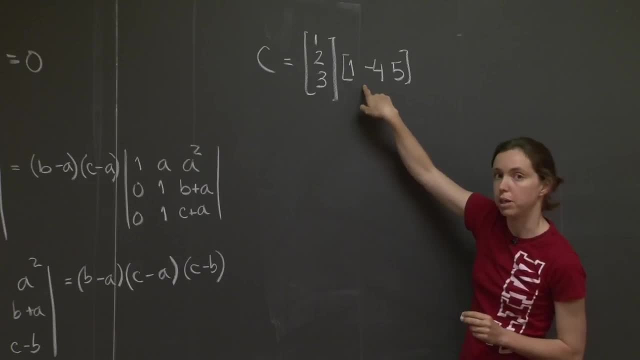 So if you write out what the matrix is, it'll be a 3 by 3 matrix, where we can think about it this way. The first row will be 1 times 1 minus 3.. 1 minus 4, 5.. 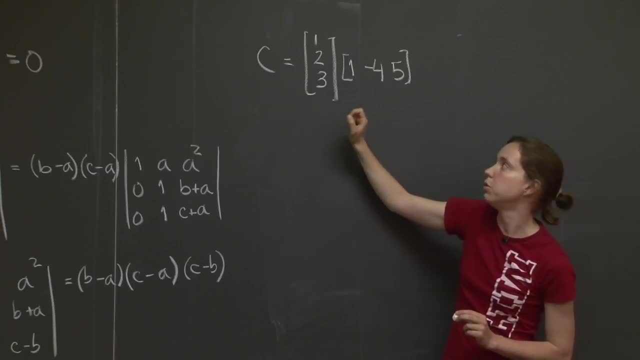 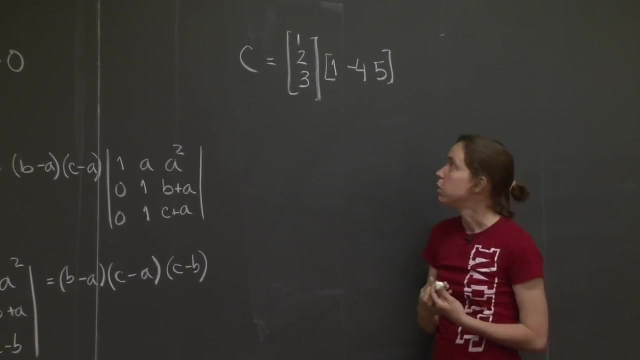 The second row will be 2 times those numbers And the third row will be 3 times those numbers. So all the rows are going to be linearly dependent, or another way of saying: the matrix is singular. When the matrix is singular, the determinant. 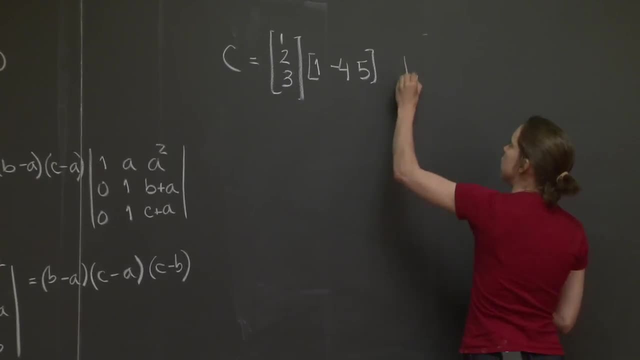 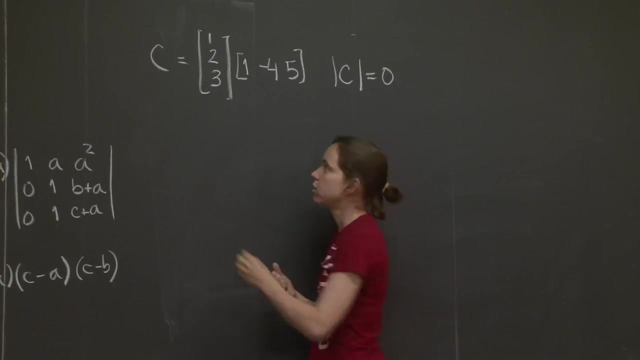 is always equal to 0.. That's also one of the properties c: 0.. On to the next matrix, last one: d is equal to 0, 0, 0.. 1, minus 1, 3, minus 3,, 4, minus 4.. 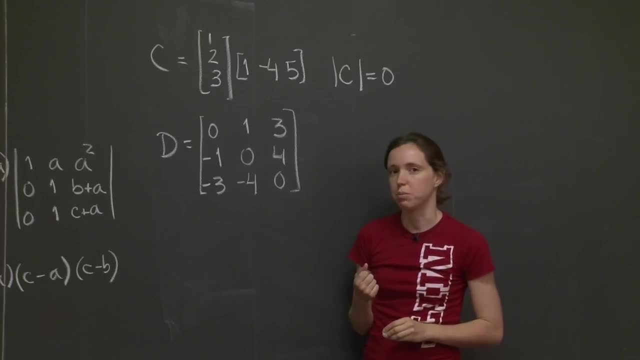 Maybe you didn't get that from just looking at the matrix in the first time, But did you see how I wrote it down? I have 0's down the diagonal And then for each entry I have minus that entry. That means that this matrix is skew-symmetric. 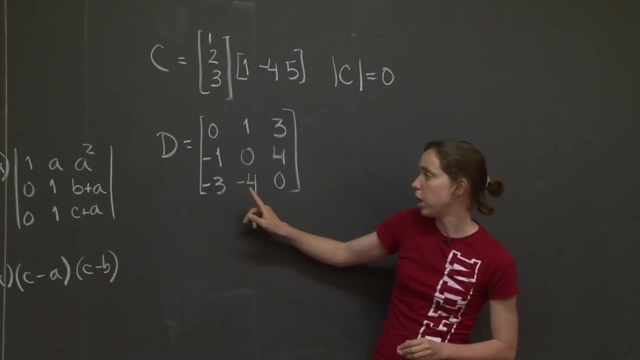 What that means is, if you do d transpose, it will not be equal to d, but it will be equal to minus d. d is equal, d transpose is equal to minus d. Now, what does this give us for determinants? Well, if these two matrices are the same matrix, 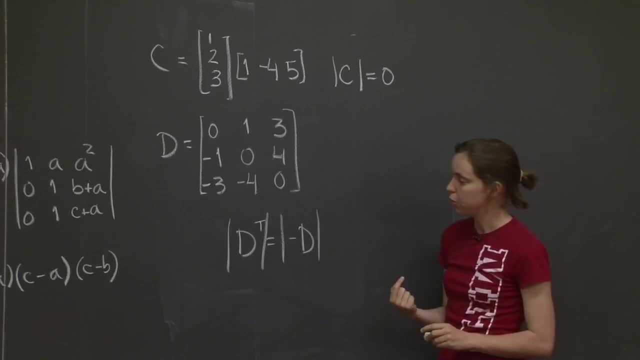 this determinant is equal to that. That's the determinant. One of the properties is that the determinant with transpose of the matrix is equal to the determinant of the original matrix. How about this side? Well, first temptation would be to just write that.